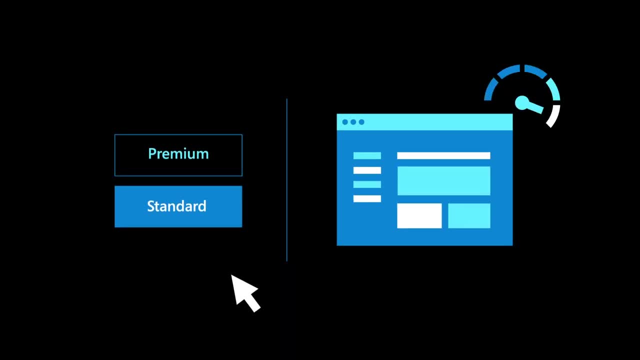 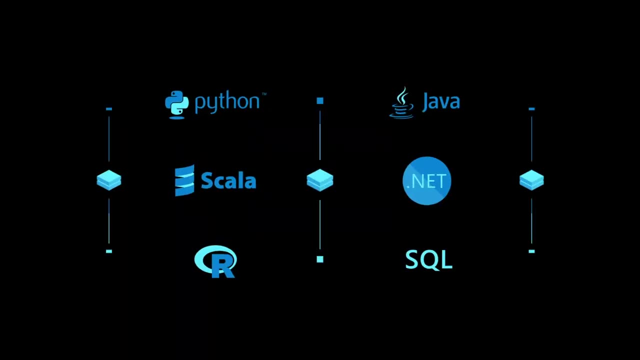 then upgrade to standard or premium for added benefits. Auto-scale and auto-termination ensure you don't overpay. The language-agnostic environment with support for Python, Scala, R, Java, NET and SQL helps you avoid retraining, Whether you're a data scientist or data engineer. 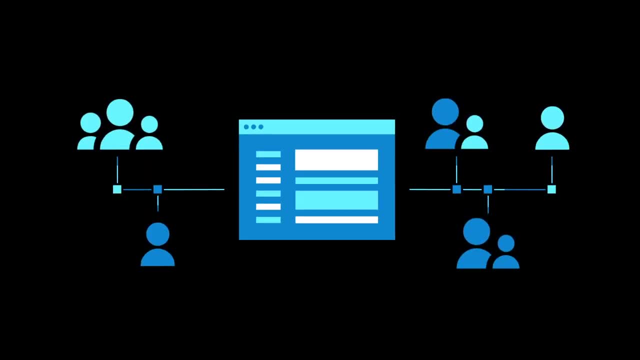 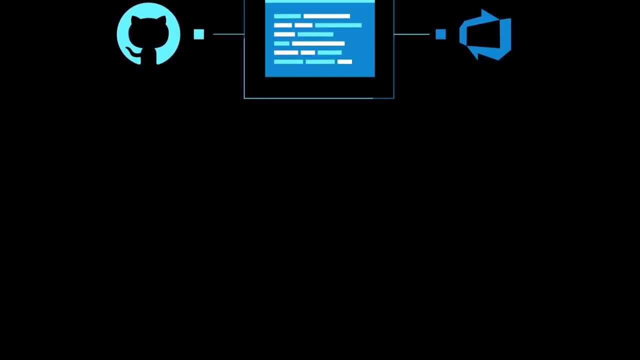 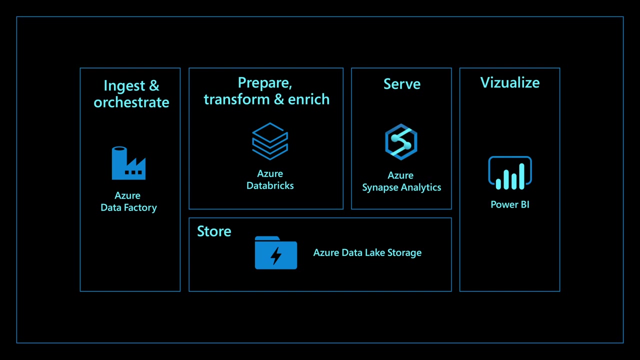 the intuitive interactive workspace promotes collaboration on a single pipeline. Get easy version control of notebooks with GitHub and Azure DevOps. Let's see it in action. Azure Databricks enables data curation and transformation for your entire data lake, so it's ready for enterprise information systems like your data warehouse or operational databases. 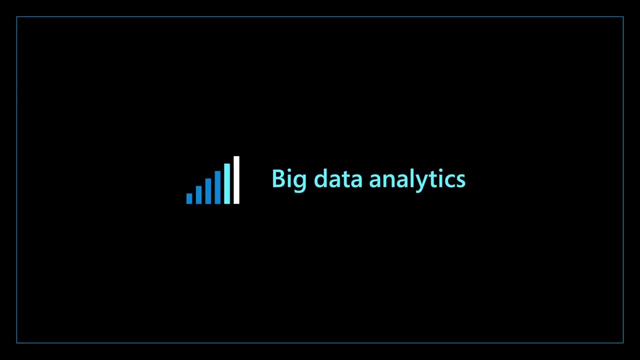 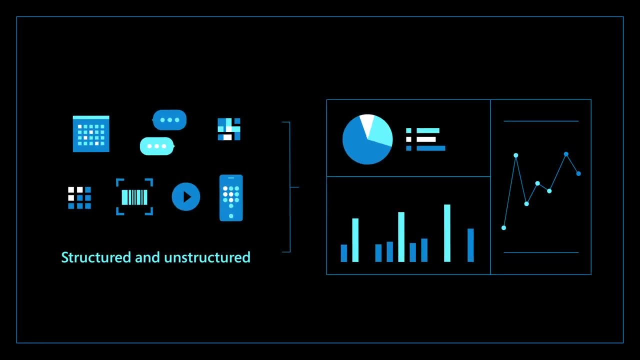 With a massively parallelized Spark engine. Azure Databricks opens up a new world of big data analytics. Extract value from unstructured and structured data alike for all your analytics jobs. But what about real-time analytics With structured streaming and managed Delta Lake? 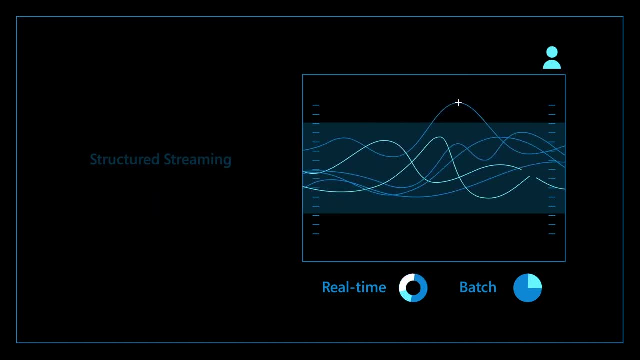 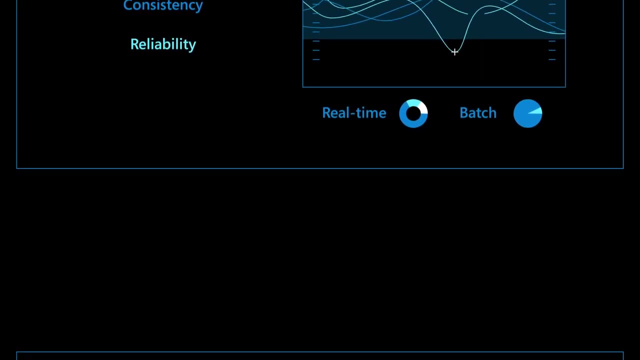 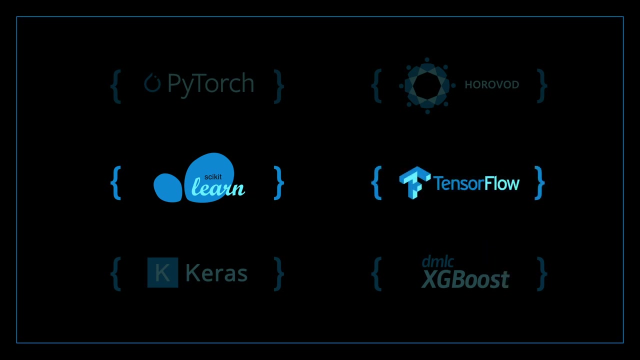 you can leverage the same data frames construct. This ensures high performance, the right level of consistency and continued reliability across your processing needs. When it comes to machine learning, pre-installed frameworks like Scikit-learn and TensorFlow simplify your pipelines. The ready-to-use environment auto-scales for fast. 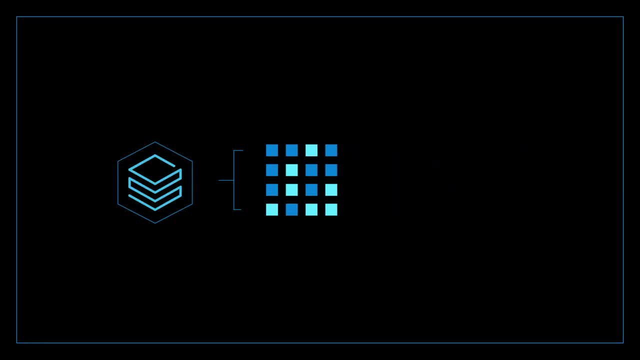 results thanks to the dedicated machine learning runtime that's built-in, And it's pre-tuned for distributed processing. Integrate with Azure machine learning to leverage automated machine learning, improve operationalization and smooth MLOps. You can also surface machine learning output into apps and reports using Cosmos DB and Azure Synapse Analytics. 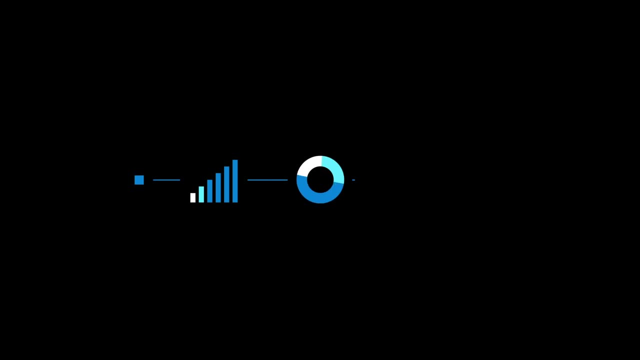 Whether you're focused on big data, analytics, real-time analytics or machine learning, you can execute any job on a single cluster. Create more efficiencies as Azure, Data, Blockchain and DevOps teams reach out to you on a larger scale than ever, automatically and intelligently creates pods of resources for each user within. 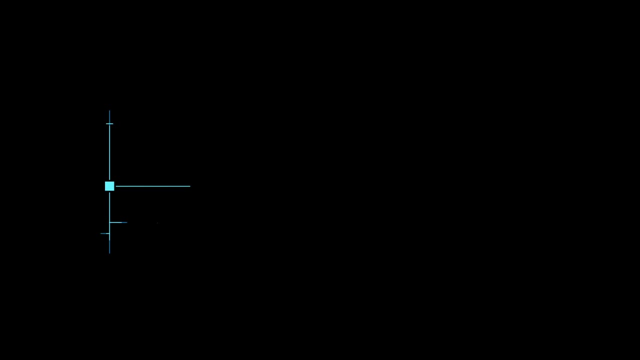 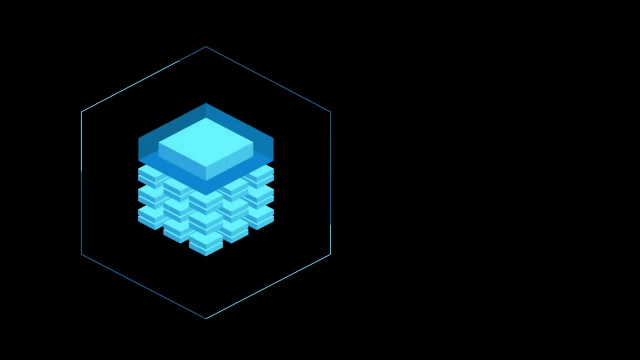 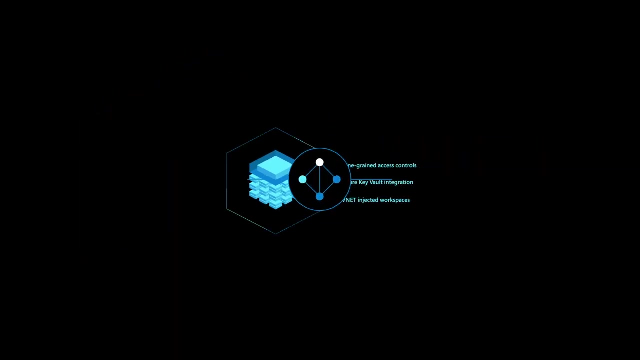 its high concurrency clusters. Native integration into the Azure ecosystem allows you to create end-to-end analytic solutions that scale with your data. Work securely with Bnet injected workspaces, Azure Key Vault integration and fine grained access controls. You can authenticate automatically with the